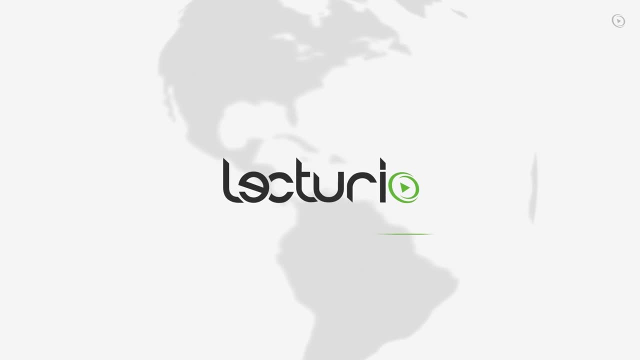 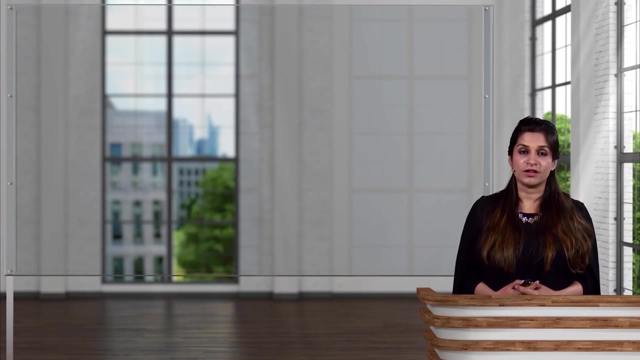 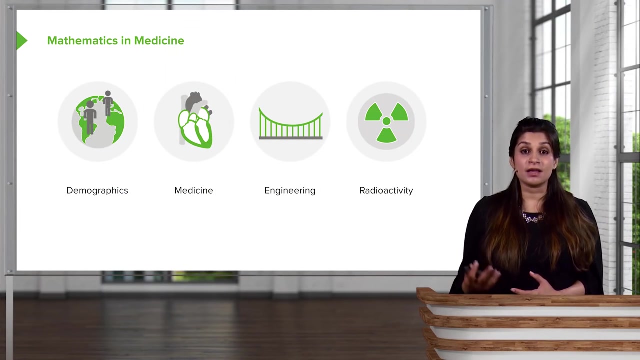 Mathematics is everywhere. If you open your eyes to it, you will start to see numbers and equations and functions absolutely everywhere. We looked at how it applies to different areas and these are just some of the main areas we spoke about Demographics, medicine. 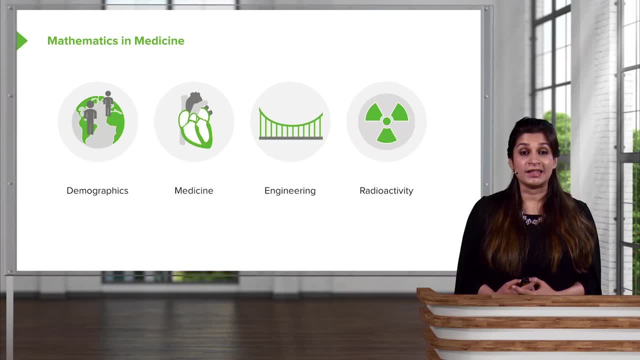 engineering and radioactivity, But now we'll focus completely on medicine. When you look at the growth and decay of any model- so look at a tumor or bacteria- you will have to use differential equations to model how they change over time. In medical imaging. mathematics is used extensively In our ever-changing world of. 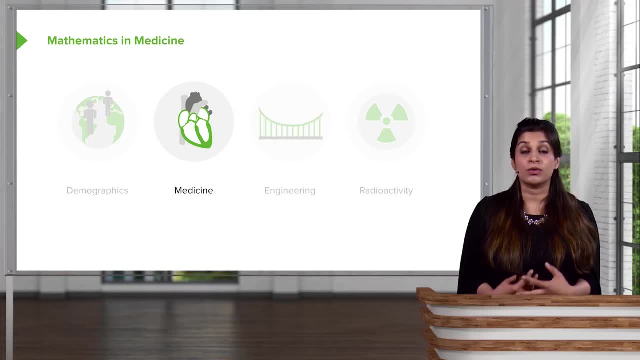 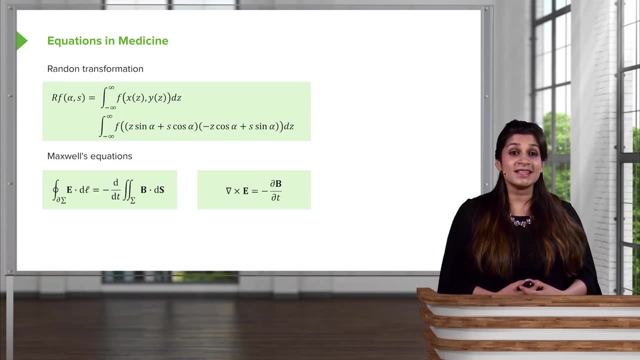 medicine, where things are becoming more technical, things are becoming more complex. the background behind it all is just mathematics. You see things like radon transformation, Which is a complicated integral equation combined together with Fourier transformations, in things like MRI scans and in ultrasounds. You see Maxwell's equation in things like 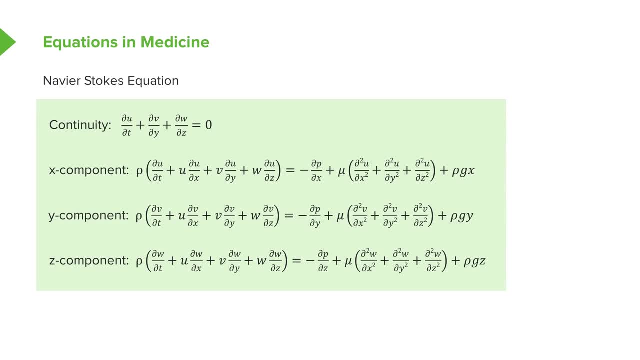 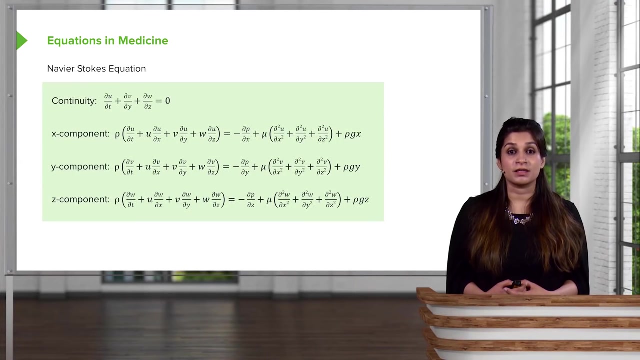 cancer, therapy of hypothermia. And the Navier-Stokes equation is just one other example of the kind of equations that we use. This describes the flow of fluid through pipes, narrow or widened pipes. You'll start to notice that these equations build the 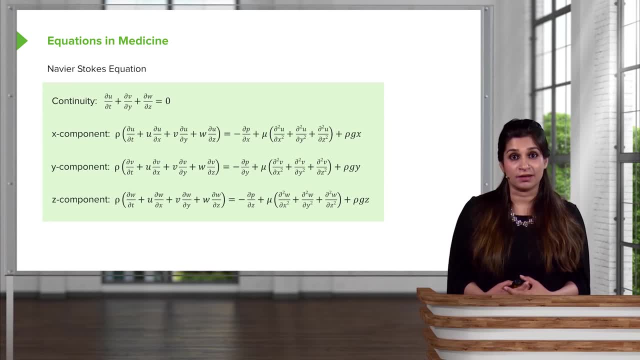 foundations of our medical study, In fact of any field, And in the modern world. You'll also see that these equations are quite a few familiar notations. You can see the integral signs, You can see the differentials, Although they are fairly complicated at this point in time. but you understand. 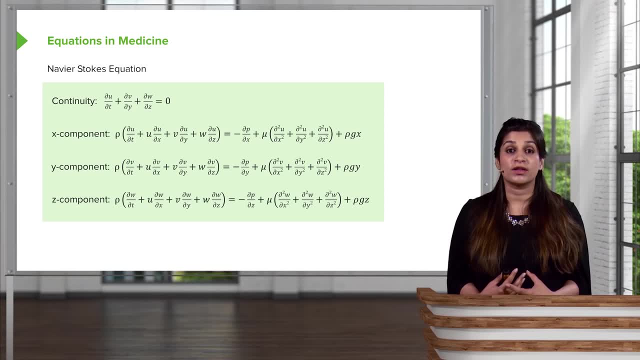 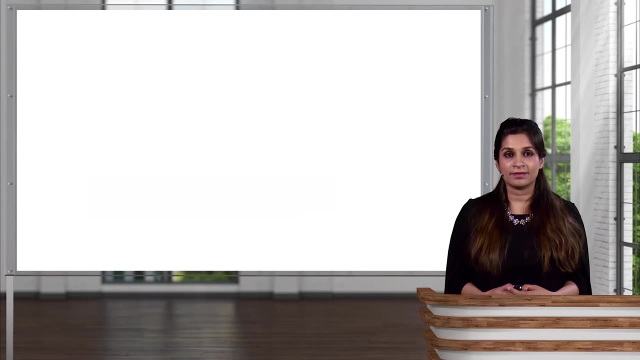 what is happening, Whether you're looking at the gradients or whether you're looking at the areas of these equations. So lets just look at some mathematical examples and see if we can apply differential equations to some real-life medical problems. Have a look at these examples. 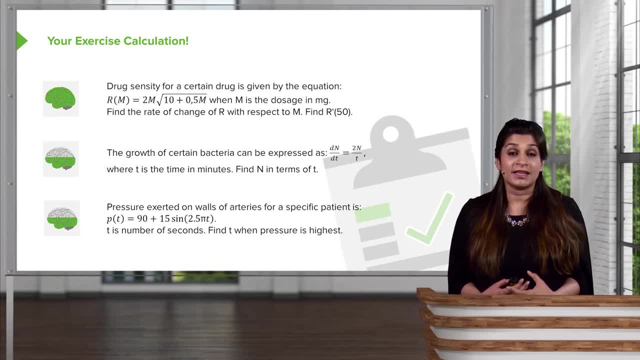 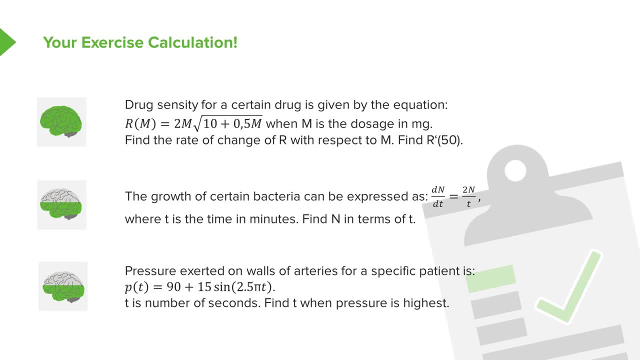 Now they're very simple basic examples and they're very specific cases that we're looking at, but it does require some use of calculus, So have a little read of them and see if you can figure these out for yourselves. We'll do them in a minute together.